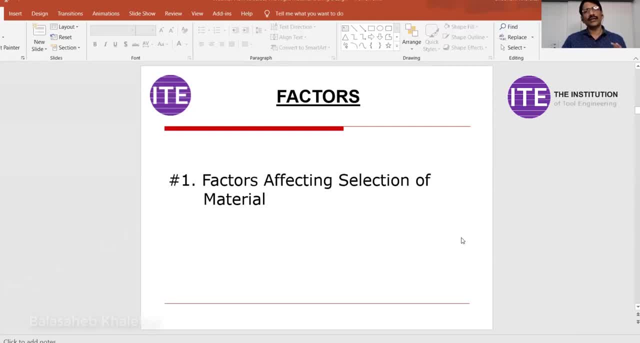 important points you think. So, one by one, we are going to understand all these factors and their relation with other points as well. First of all, we have to understand what is my requirement. If you are designing a product like, say, engine mounting bracket, you have to understand. 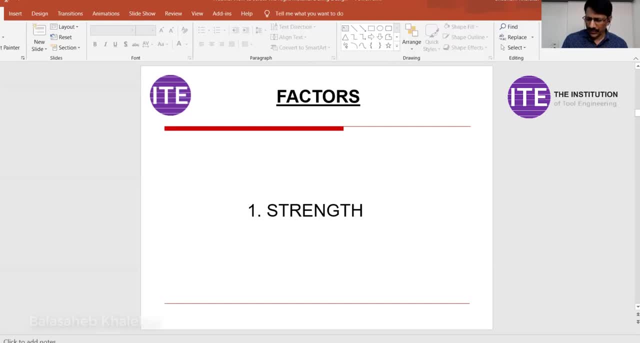 which are those failures that may occur. So, whether you have to go for a tensile strength that is more important or you have to go for a tensile strength that is more important. So, whether you have to go for a tensile strength that is more important or you have to go for a 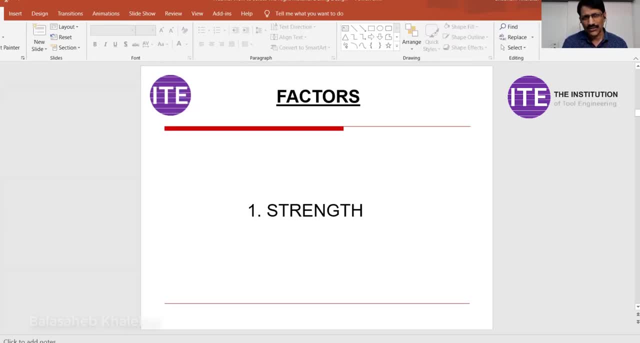 compressive or shear strength, that you have to understand And as per that you have to select the right material. So you have to consider other factors as well. So when you want to go for a better strength, other elements are also important, like hardness- then alloying elements right. 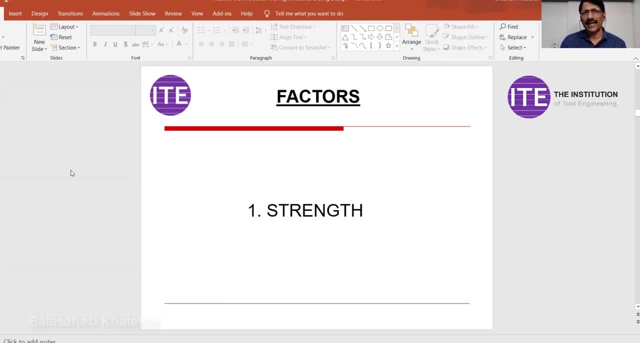 So when strength is important, then you may have to go for a material like steel or you may have to go for alloy steel. we can say: In that case other materials will not work. So we will understand. it is a vast subject, friends. Right from we can say: 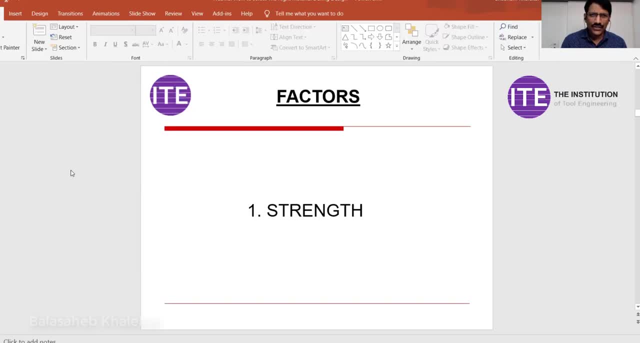 wooden material, then thermoco. these are all engineering materials: rubber, plastic, steel, aluminium. these are different kinds of materials And I am going to give you some cool tips today how to focus on which materials. So, one by one, we are going to understand all these points. 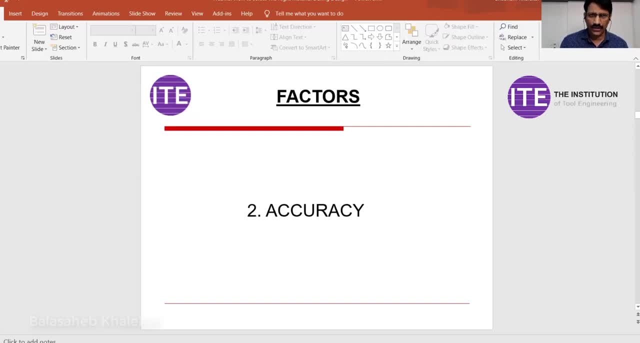 Second point is the accuracy. What is that accuracy you want to achieve? If you are saying your accuracy requirement is, say, 5 microns or 2 microns, rubber material will not work, wood or material will not work. you have to go for a steel or say aluminium. So once you understand, 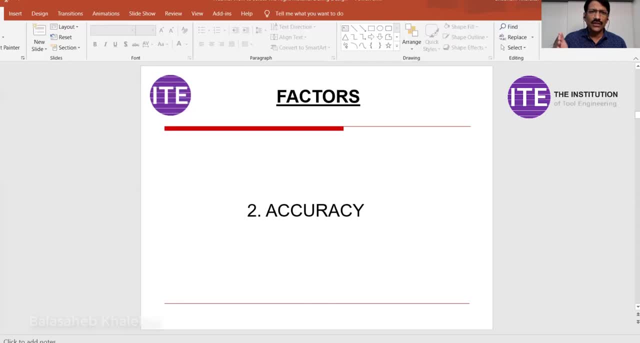 the strength factor, then you have to understand what is that accuracy you want to achieve? Now, there are three terminologies here. One is tolerance, second is accuracy and third is quality. They are similar terminologies. Tolerance is specifically to the dimension and geometry. right, We say geometric tolerance. 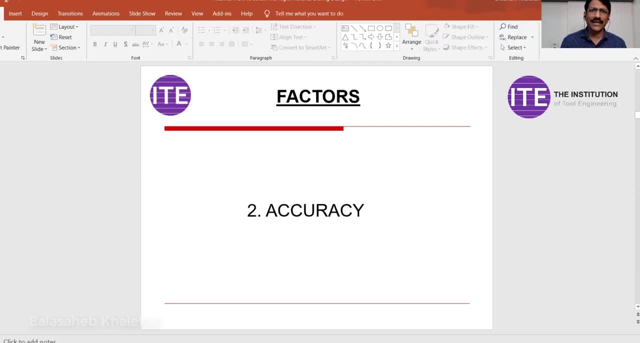 or we say dimensional tolerance, But accuracy can be related to dimension, maybe related to speed, temperature, velocity. And when we say quality, quality is a broad perspective. Customer satisfaction means quality, but they are very similar. So we have to understand what is my requirement And if you are designing, say, die or tool, 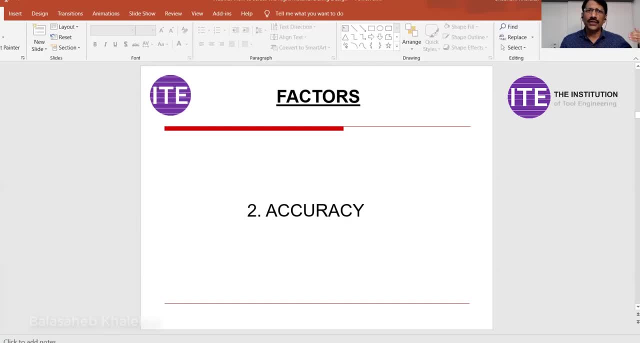 you have to understand what is that accuracy you want to produce on the component. Then, third important factor: cost. yes, very important part And during interview- designers interview- this is one important question- generally asked how you will reduce the cost of this product. Imagine you are a design engineer and you are working in the product. 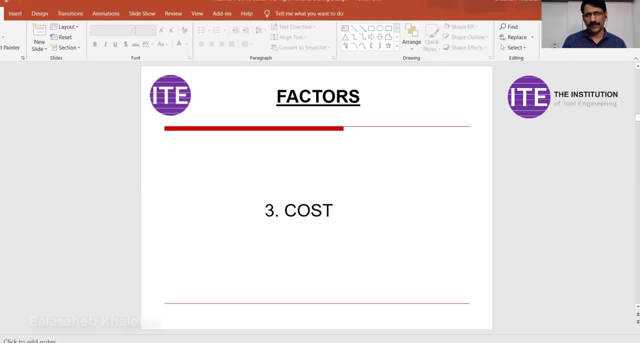 design field. how you will reduce the cost of your product. have to purchase a laptop, so the first thing is all about your budget, cost right. then you will think about other parameters. so which are those important points? how you are going to save the cost of your product so you can change the material, and who will help you in this purchase. 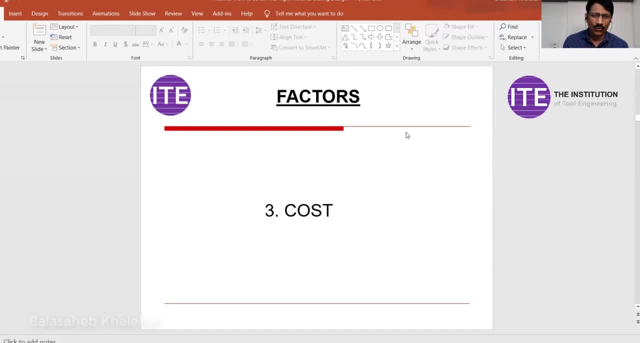 engineer earlier days, maybe 20, 25 years back- what was the situation? design engineer will design as per his knowledge, he will release the drawing and there are so many problems during manufacturing, assembling and proving of the product. but nowadays there is a concept called as a pre-en concept. 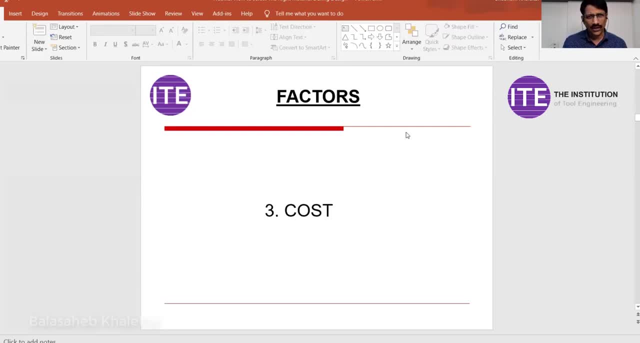 pre-en means en means engineering. notice means before releasing the drawing. there is a cft, that is, cross-functional team, and you are discussing your design will with all these team members. and who are the team members? one is from production, production, quality, marketing, purchase, service, materials department. all these people will be there. 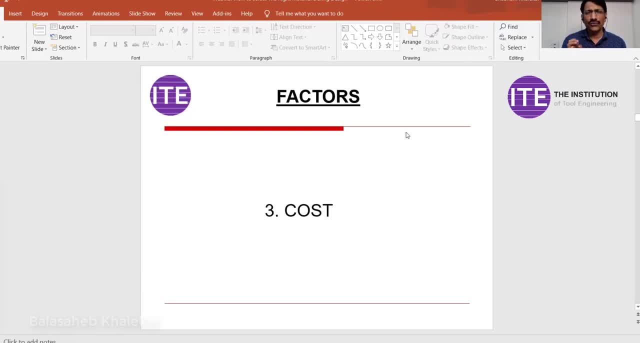 in your team. so purchase engineer is the person who will guide you regarding material, because he is every day in the market and he will suggest some good material. he will say that put this material because this is less costly and giving the same strength or quality. that is value. 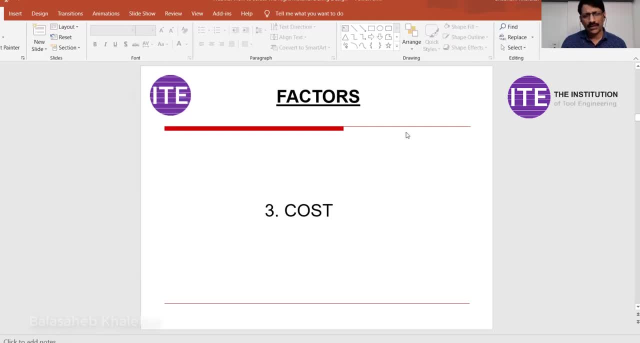 engineering. value engineering means you are improving the quality of the product, keeping the same cost, or you are reducing the cost of the product, keeping the same quality. that is value engineering. and one way is to change the material. another way you can change the process. if the component is produced by forging, you can produce it by casting. if it is produced by casting, 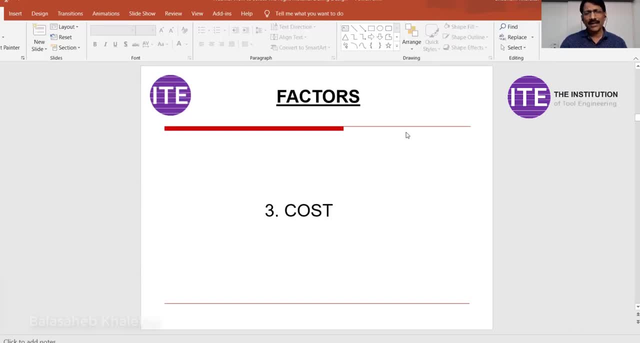 it can be produced by sheet metal. if it is produced from sheet metal it can be produced from plastic molding. so if you are changing the process, then also you can reduce the cost of the product. then you can simplify the design means number of- we can say size. you can reduce number of parts you can. 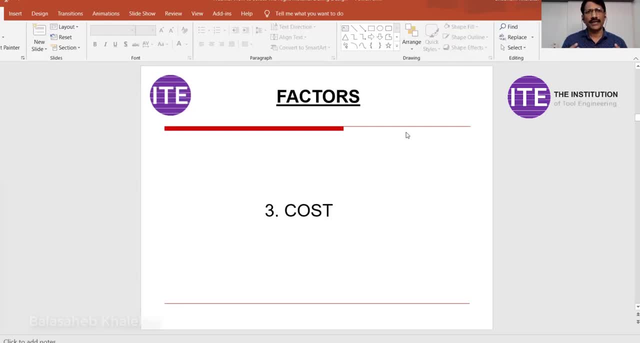 reduce. so if it is a, say, steering gearbox geometry, steering geometry right from steering wheel up to between steering wheel, up to steering wheel, to tyre rod and steering knuckle, suppose there are 10 Opening components, can you simplify and make this design by using seven components? that should be your approach. Then you can go for resizing it. sometimes you can delete the part as 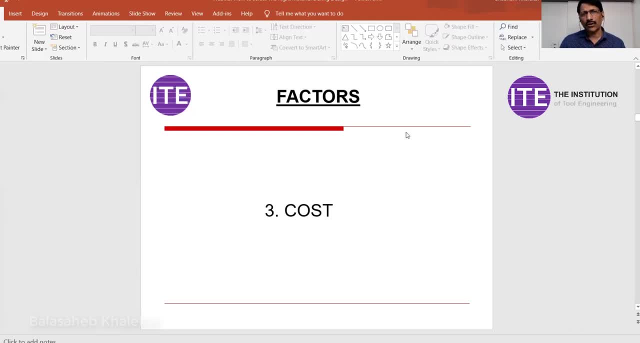 well, that is also the possibility, because if you consider the product like a car, there are thousands of products. that means components are there. four thousand, five thousand components are there and sometimes there is a possibility that part may not be useful. that also you have to understand. Coming to the next point: quantity. 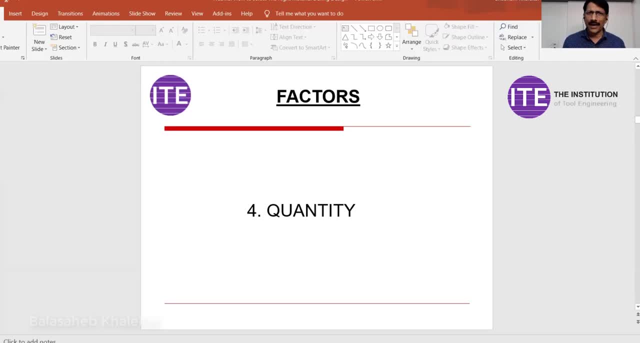 what is that quantity you want to produce? So if it is for prototype activity, you can go for different material. If you want to produce thousands of components, lakhs of components, the material could be different. Say, let us take one example of say: 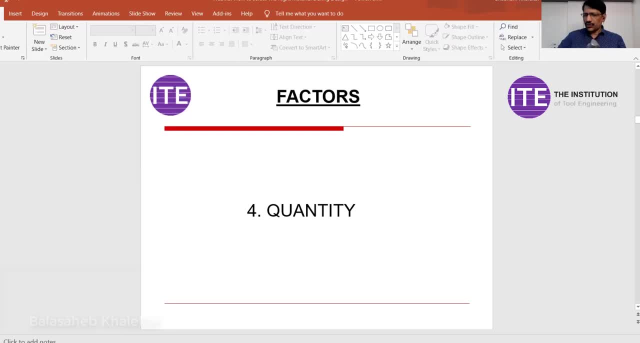 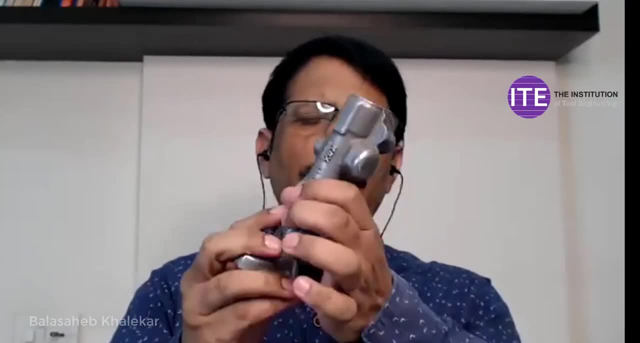 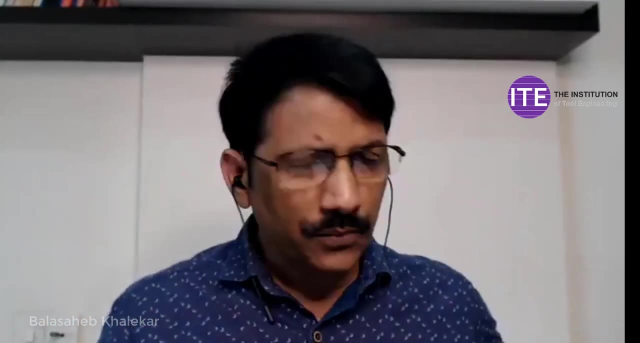 aluminum, So I have one component here. I can show you this. So if you understand, suppose you want to produce 10 components, So I have one component here, So you can go for the process like sand casting. But if you want to produce, say, 1000 components or 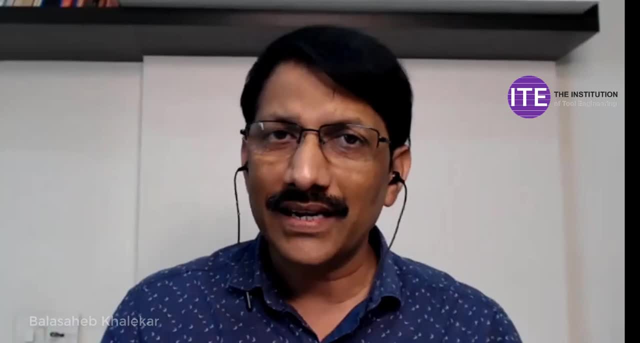 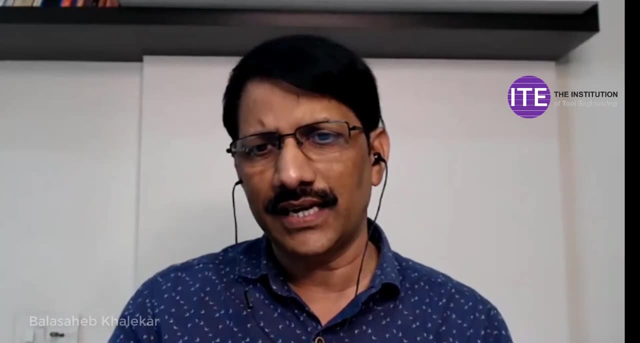 10,000 components, then the process could be die casting. Now, as per that, different, different processes are also there, like PDC is there, GDC is there. So again, which process you want to select, that also you can go for. So if you want to produce 10 components, 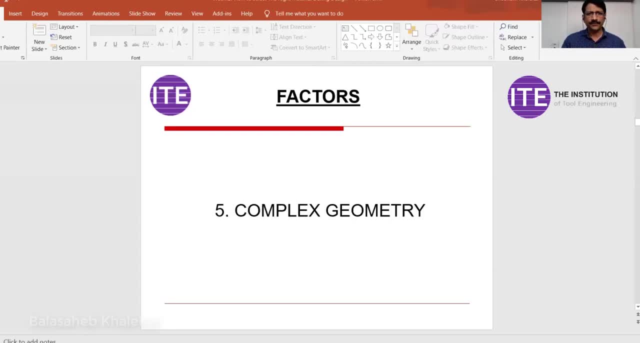 also depends upon this. Next point: complex geometry. very important. Design engineers should understand what is that material that can produce such type of complex geometry. say aluminum, Aluminum material. what is the property of aluminum material? Excellent castability property. So here we have to understand various properties of material So it can take. 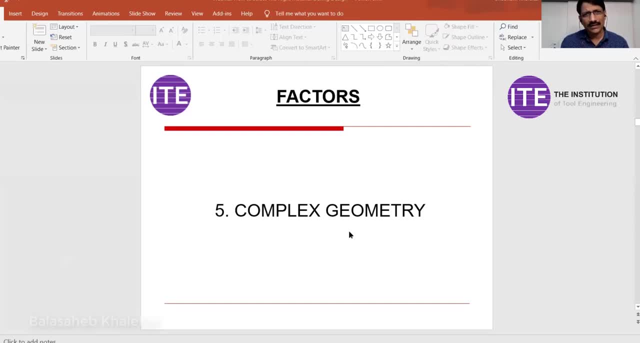 any critical shape. Same is the case of cast time. the name suggests that casting It can take any critical shape. So when there is a possibility of critical shapes you can produce by using aluminum or cast time or SGI and to some extent steel, because still generally casting. 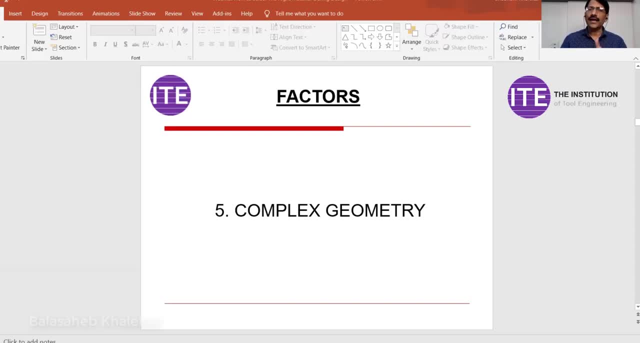 difficult to produce. There are some defects, are there that we have to understand. So, when you are designing your product and when you are focusing on the shape, you have to understand the limitations about the materials- different, different materials- And therefore you have to. 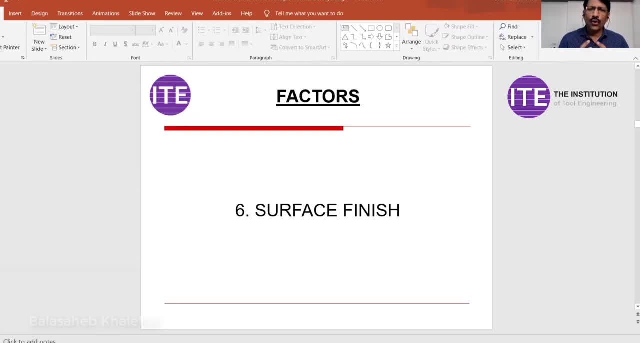 understand the possibilities. Next point is surface finish. What is that quality you want to achieve on the product? If you want to go for a three triangle, that is, we can say 0.8 microns, then the material could be aluminum or steel. So requirement of surface finish, and what is? 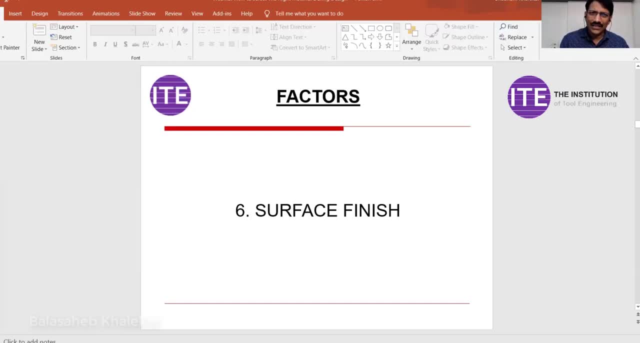 the possibility about that material. that study is very, very important. Coming to the next point, size of the part. You want to produce a component of 2 gram, 2 gram component. then the material it is very difficult to machine right. So you have to go for different, different processes, Like you can go for. 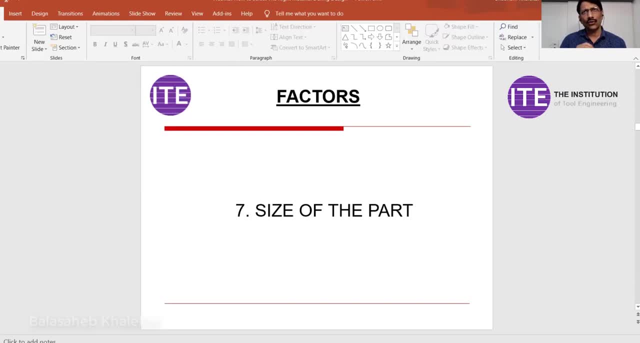 investment casting process. So investment casting process, then only steel alloys. some certain steel alloys you can produce. For example, if you want to produce a components of, say, size 8000 mm, then you have to go for a different material. Definitely you can produce by using cast time. 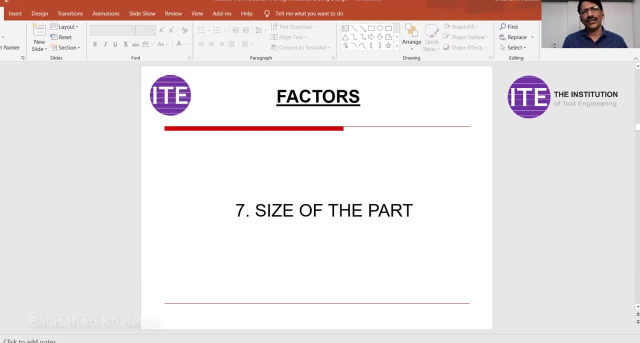 So as per the size, again, limitations are there In such cases. rubber material: you cannot produce that component Like plastic. you will have some limitations that we have to understand. Then machine ability: If the component material is cast time it is giving good machinability compared to steel. Means machining time. also you have to cast time. If the component material is cast time, it is giving good machinability compared to steel. Means machining time. also, you have to cast time. If the component material is cast time, it is giving good machinability compared to steel. 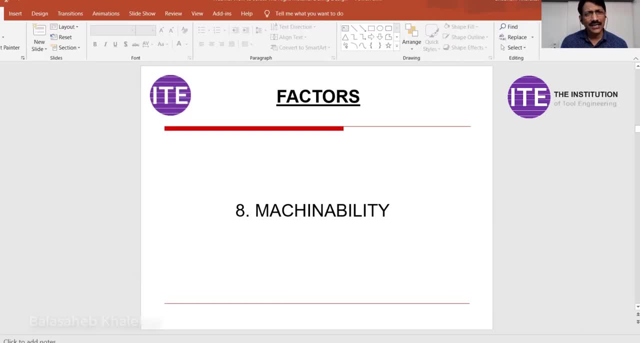 Meshing time. also, you have to consider in such cases, Aluminum, excellent machinability property. So, as per the material, this property, you have to understand which has better for me. So, as per the material, this property, you have to understand which has better for me. 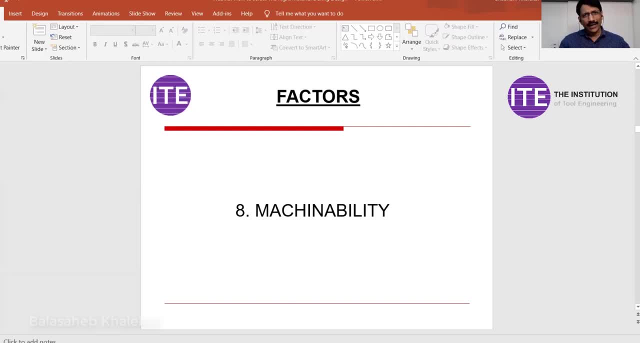 and it is not dependent only on one aspect or factor. sometimes holes in the material, and it is not dependent only on one aspect or factor. sometimes holes in the material, factors also you have to consider and it should be a conscious decision. Next point is of the Manufacturing product. 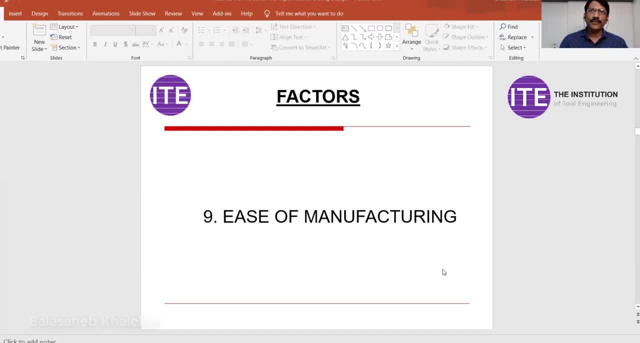 this is called Dfm. This means the material while we run a space moving won't receive. Suppose the geometry is complex and you want to go for a particular machining process. Imagine there is a slot of width, say 2 mm width. length is, say, 10 mm and depth is, say, 6 mm. 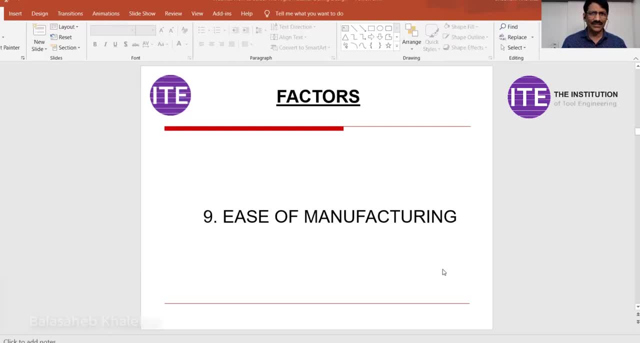 That is a cavity you want to produce. So in such cases it is very difficult to machine it right, So you have to go for EDM, that is, electro discharge machining. So in such cases if the process is changing, then the material should be as per that, because 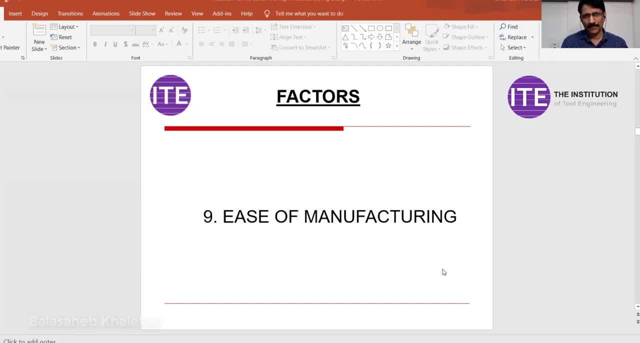 other materials, EDM process is not possible. Another point: sometimes it is not possible to machine that particular feature, So you may have to go for designing of the insert. Insert means a separate piece. you are fitting in that particular die or assembly so that 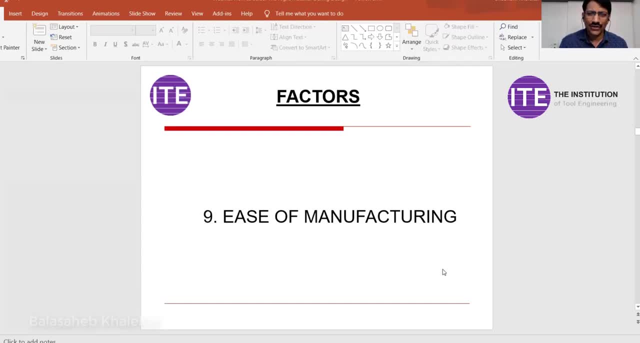 you can achieve that And design for manufacturing. So insert means separate piece, you are machining and you are going for the fitment. So in such cases also you have to understand other factors. Is this possible, So that flexibility should be there if you are using a particular material? 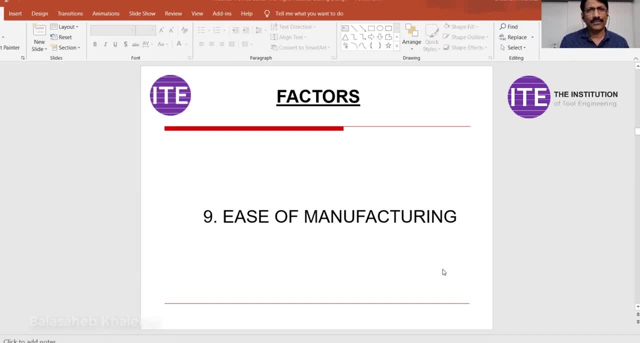 So if it is a cast tile and if some changes are required, then you cannot go for welding, because that is, we can say, the appearance will be affected, customers dissatisfaction will be there. all these aspects could be there. Coming to the next point, ease of modification, that we have to understand. if some changes 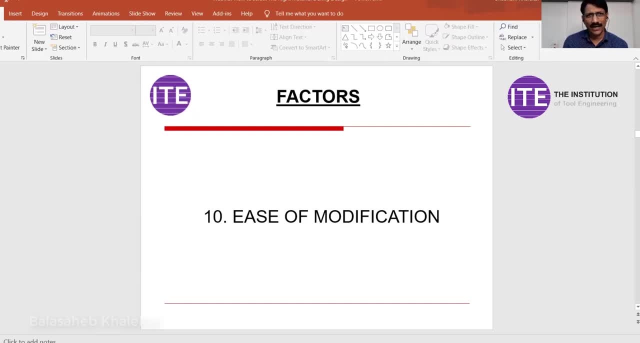 are there in the product design and you are receiving the drawing from R&D as per that, you have to go for some modifications. So how it is easy, if you are using this particular material, that flexibility, you have to go for this review. Next point: weight. 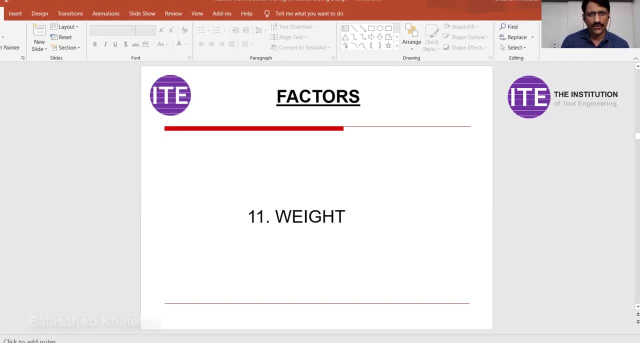 Now this is one constraint when you are going for some conventional methods like, for example, handling Handling. So if there is an issue in such cases, then weight is the constraint. So, like cast time or steel, the density say 7.8 gram per centimeter cube. 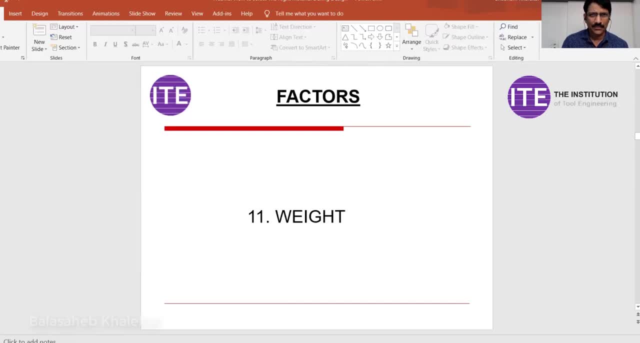 So in such cases can you go for lighter material like aluminum or rubber or plastic, that you have to understand. So product design engineer or tool design engineer has to understand all these aspects as per the different, different, we can say- achievements. Coming to the next point, life. 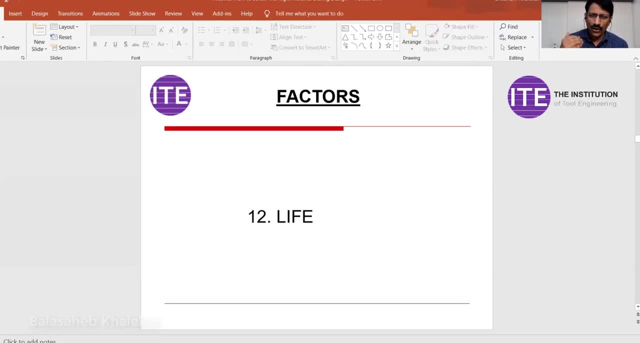 What is that life You want to achieve? and for this you have to understand the life cycle of that particular product. Some components or products life cycle may be 20 years, 30 years, Some products 3 years, 4 years, Some products may be few months, as per that, material will change and how you will understand. 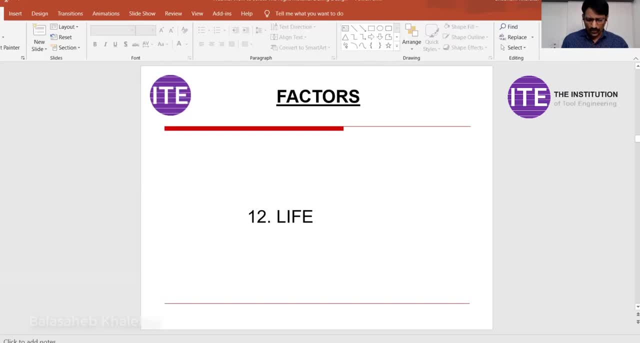 this. This is again a design input, So if you are working in design department, you have to ask this question to your company Customer: what is that requirement, as per that, you can select the right material. Coming to the next point: availability. 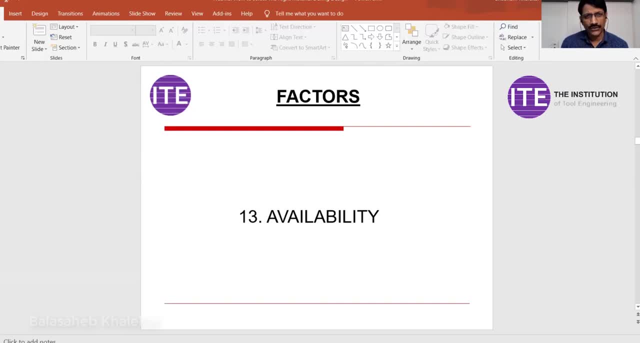 Right. So, even though this is not a technical point, but you have to consider in COVID situation, sometimes it is not possible that it is available in the market, So you have to go for alternate material. that purchase engineer can guide you about that. 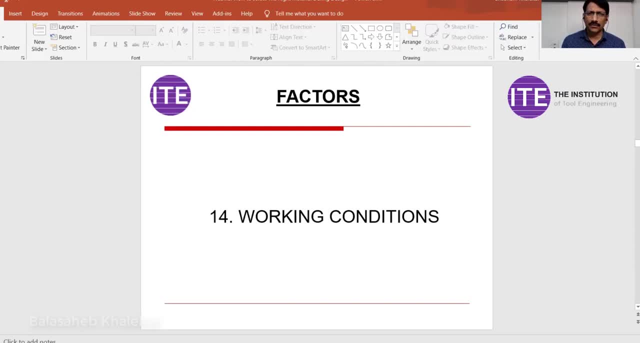 Next, working conditions. Working conditions like temperature pressure. as per that, Sometimes, if the temperature Temperature is very high- plastic component or rubber component- there is a possibility that it cannot function. then you have to go for different material. Then that is a lower condition. as per that your material will be changing. 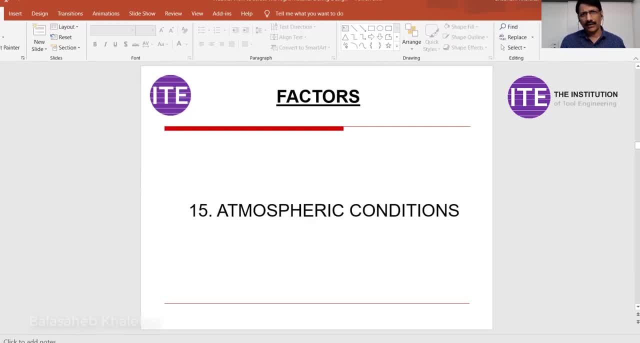 Then atmospheric conditions. suppose you are designing a car and the car can be used in different different states: Jammu and Kashmir, Rajasthan, Chennai area or Tamil Nadu. So if temperature conditions are different or atmospheric conditions are different, Then what is the effect on that particular material? that also you have to understand.